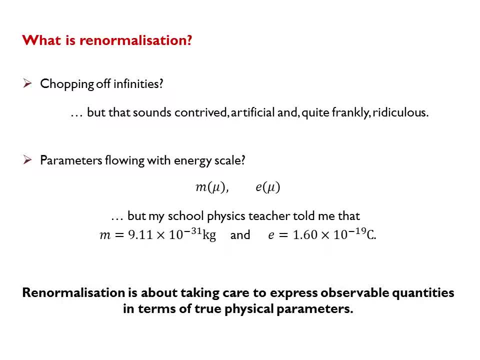 Any infinities that arise are not a fault of quantum field theory itself, but are due to invalid reasoning by the person doing the calculation. 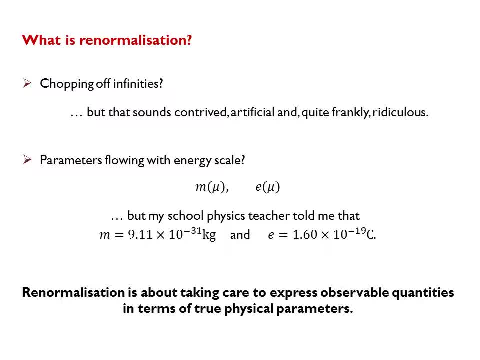 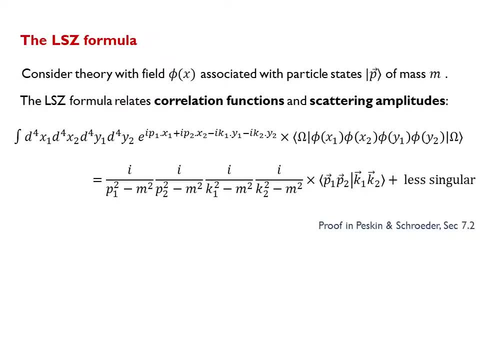 that we memorized at school. 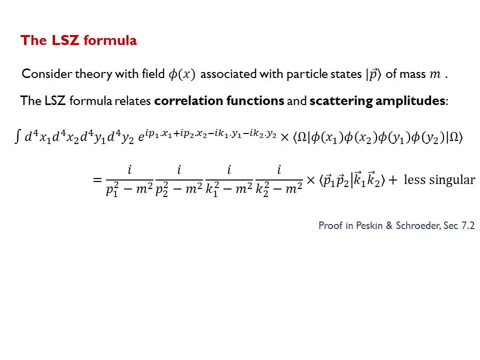 Since renormalisation is all about making sense of physical observables, I have to start this talk by describing how physical observables are computed in QFT. 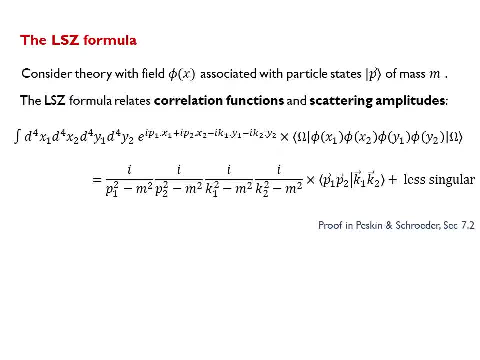 And the key equation is something called the LSZ formula. The LSZ formula is a bridge between what theoreticians can calculate and what experimentalists can measure. 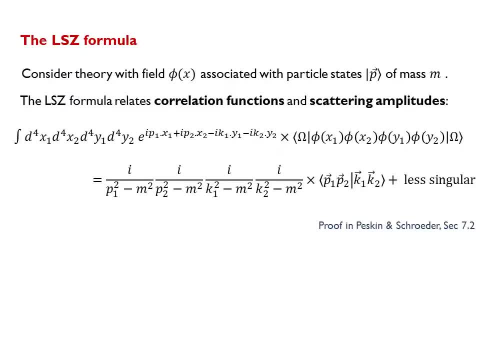 This formula tells us how to convert correlations into equations or equations where a corresponding correlation functions which can be computed using Feynman diagram technology into scattering amplitudes which determine the outcomes of particle accelerator experiments. It says that the Fourier transform of an endpoint function has an nth order pole in momentum space and the residue of this 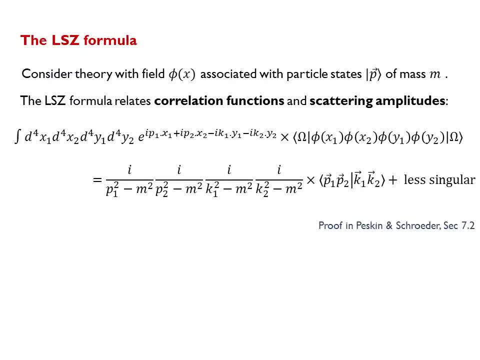 pole is precisely the scattering amplitude for the corresponding scattering process involving n particles. In other words, a Feynman diagram calculation of a correlation function can be converted into a quantity that can be observed in real life. 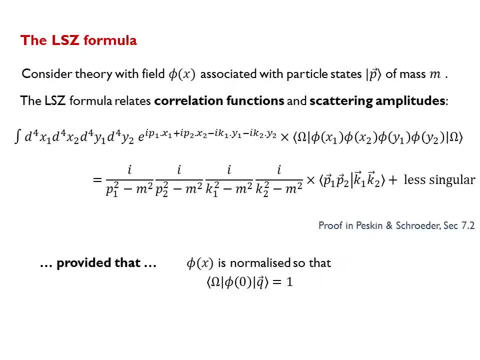 This formula can't be applied carelessly because it comes with a condition on how the field is normalized. The condition is that the field operator acting on the vacuum state creates particle states with unit norm. It is easy to see that this normalization condition holds automatically in a free theory, but it's not guaranteed to hold in an interacting theory. 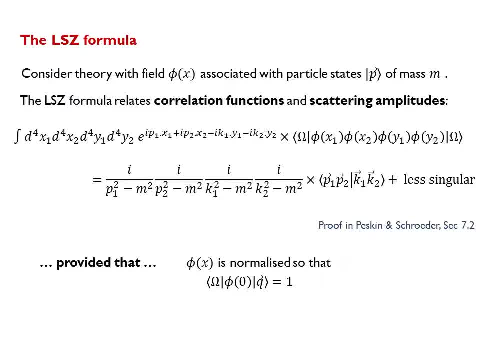 It's not guaranteed to hold in an interacting theory. If the normalization condition does hold, then great! You can go ahead, compute an endpoint function, plug it into the LSZ formula, and get a scattering amplitude which you can observe. If not, then before you can use the formula, you have to adjust the normalization of the field. In other words, you have to re-normalize it. 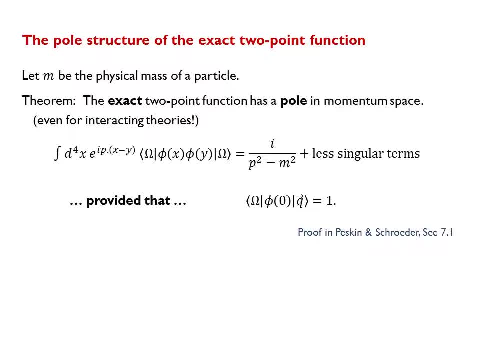 So the all-important LSZ formula comes with a condition on how the fields are normalized. Am I right? 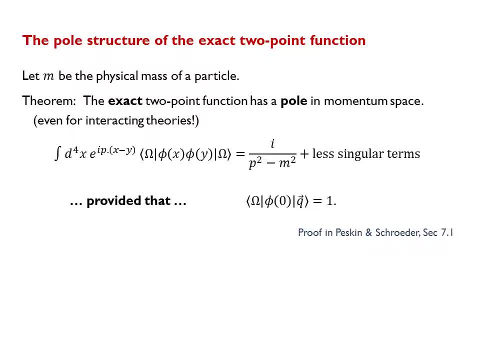 Is there an easy way to check whether this normalization condition is satisfied? There is a way, and the place to look is the exact two-point function. 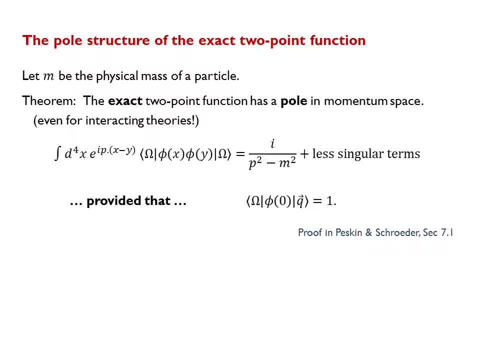 In a free theory, the exact two-point function takes a very simple form. It's just i over the momentum squared minus the mass squared. 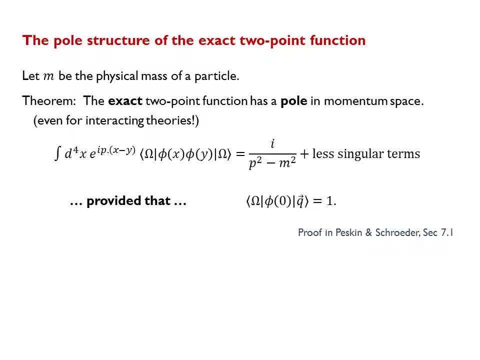 But in an interacting theory, the exact two-point function is a very complicated quantity dependent on many different Feynman diagrams. However, there's a errors in this example! 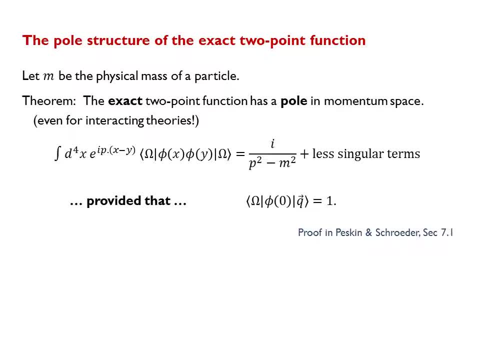 two-point function always has a pole, and the position of the pole is the physical mass of the particle in the theory. And also, provided that the LSZ normalisation condition is satisfied, the pole has residue 1. So if you want to check the LSZ normalisation condition, you could compute the exact two-point function and see if it has a pole with residue 1. Should the residue turn out to be something else, then you must adjust the normalisation of the field before using LSZ. And as a bonus, the pole structure gives you 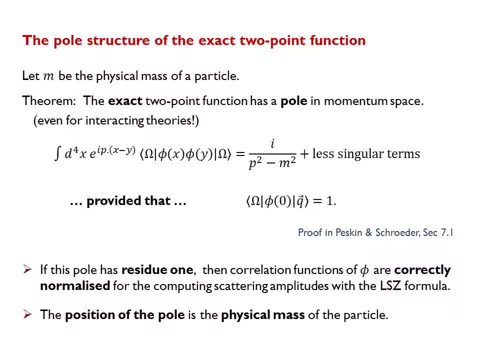 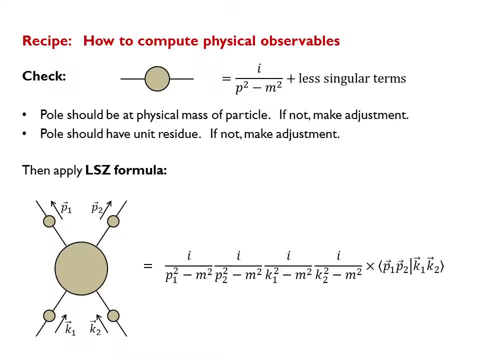 a second piece of useful information, which is that the position of the pole in momentum space is the physical mass of the particle. So if the mass parameter that you're using in your calculation fails to coincide with the position of the pole, then you must adjust the value of your mass parameter before doing anything else. 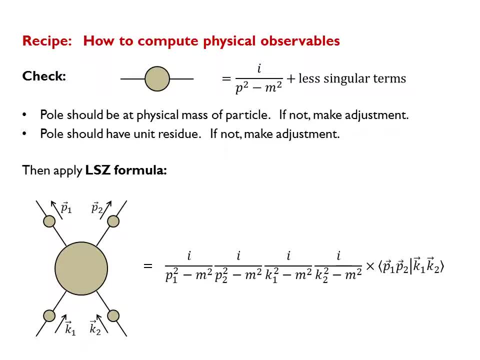 We now have a two-stage recipe for computing physical observables in QFT. Subtitles by Simon Shuel The first thing you must do is look at the pole structure of the exact two-point function. 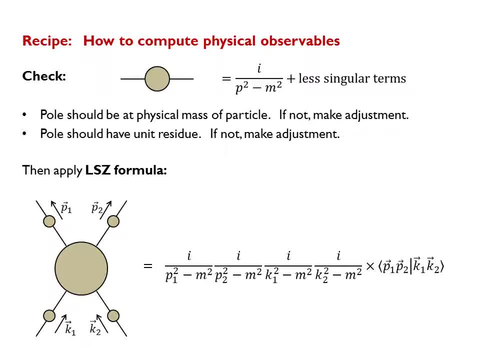 If the pole of the two-point function doesn't coincide with your mass parameter, then your mass parameter needs adjusting. And if it doesn't have residue 1, then the normalisation of the field needs adjusting. Only after you have made those adjustments can you legitimately apply the LSZ formula to convert Feynman diagrams into observable scattering amplitudes. 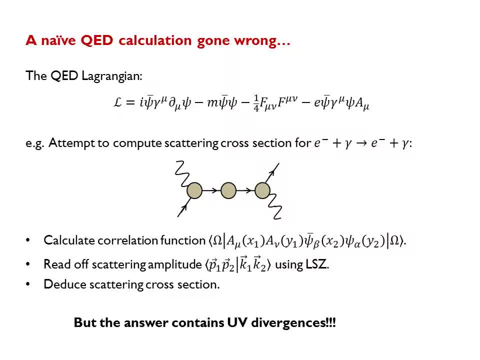 Now, let's put this into the context of QED. A typical QED quantity that we might be interested in calculating is the cross-section for the scattering between an electron and a photon. The LSZ formula tells us what to do. We have to calculate the correlation function for two gauge fields and two fermion fields. If you immediately put this correlation function into the LSZ formula, your scattering amplitude would have divergences. But that's not because there's a problem with QED! It's because there's a mistake in the calculation, and the mistake is that we skipped the first half of the recipe. We haven't done the checks and the adjustments that are required in the beginning. 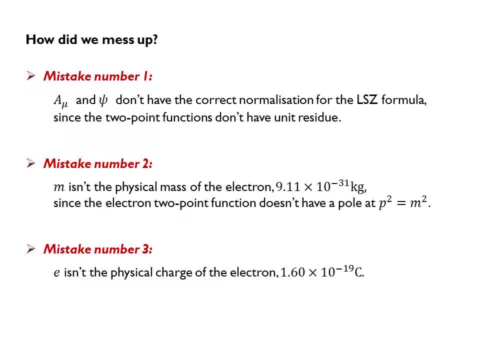 In fact, we are guilty of making three separate mistakes. The first mistake is that the fields in the Lagrangian are not normalized properly. We could have spotted this if we took the trouble of examining the residues of the poles of the two-point functions. The second mistake is that we ought to express the scattering cross-section in terms of physical parameters. But the mass in the Lagrangian is not the same as the physical mass of the electron. The mass in the Lagrangian is only the pole in the free propagator, whereas the true mass of the electron is the pole in the interacting propagator. And the third mistake is that the charge parameter in the Lagrangian isn't the same as the physical charge of the electron either, and I will have to explain why. I will explain this in more detail later on. 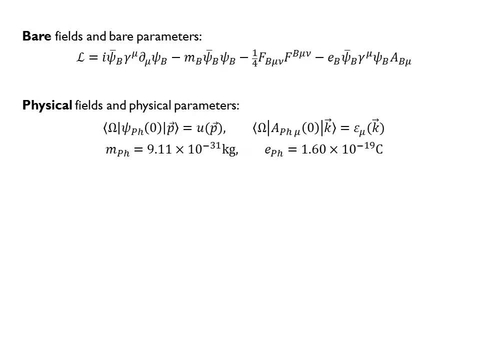 To do this calculation properly, we have to distinguish between two types of quantities. We have to distinguish between the bare fields, which are the fields in the Lagrangian, and the physical fields, which are properly normalized versions of them. We also have to distinguish between the bare parameters, which are the parameters in the Lagrangian, from the physical parameters, which are the parameters whose values you can find in formula booklets. And we are going to give names to the differences between the bare and physical parameters. We are going to call them the counter terms. Delta A, Delta Psi, Delta M, and Delta E. 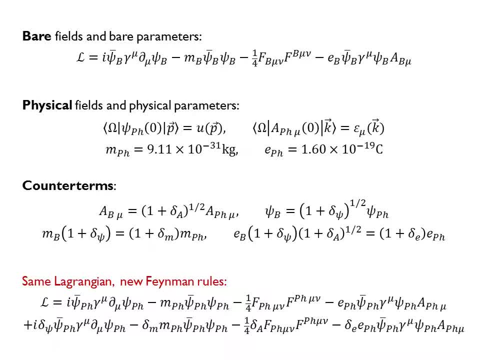 Having defined the counter terms, we are going to write out the Lagrangian again, this time in terms of the physical fields and the physical parameters. There are going to be extra terms in the Lagrangian explicitly involving the counter terms, and these are going to give us a number of terms. 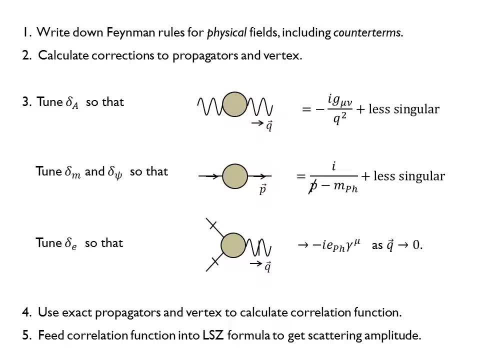 This is the accounting procedure that we are going to follow. First, you write down the Feynman rules for the physical fields, including those extra rules that involve counter terms. 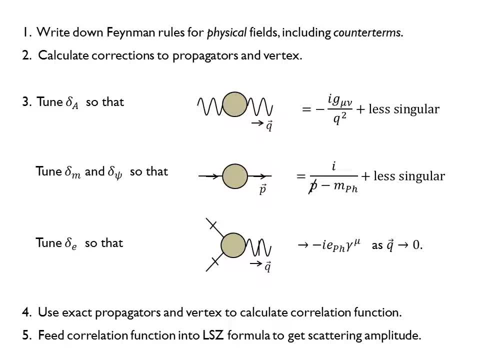 Then, using these Feynman rules, you calculate corrections to the QED propagators and the vertex to whatever order in perturbation theory you require. 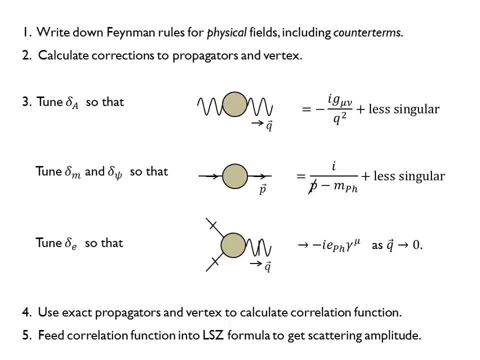 Now comes the crucial calibration step, where you tune your counter terms to the QED propagators, in such a way as to ensure that your physical quantities are normalised in the way that you want. 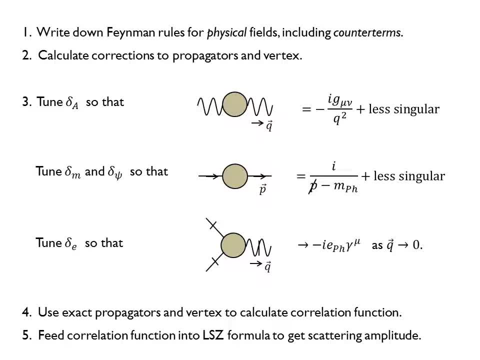 For example, in order that the photon field is properly normalised, you must tune the Delta A counter term so that the photon propagator has a pole of residue 1. 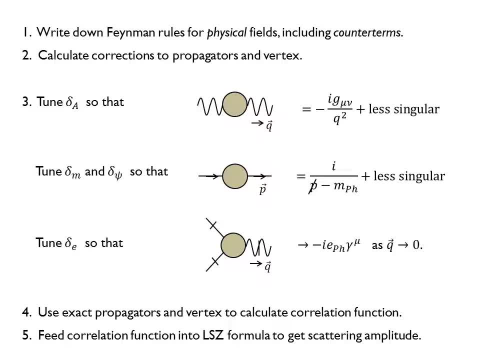 Similarly, the electron propagator must have residue 1 to guarantee that the electron field is properly normalised, and the pole must be situated at P slash equals M physical to guarantee that M physical will be normalised. 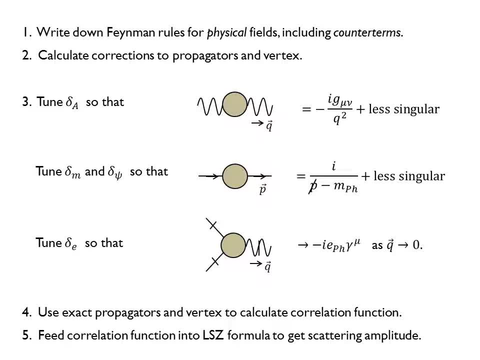 Finally, you have to find out what is the true physical electron mass. You have to meet both of these requirements at the same time, and you do so by tuning the two counter terms together. 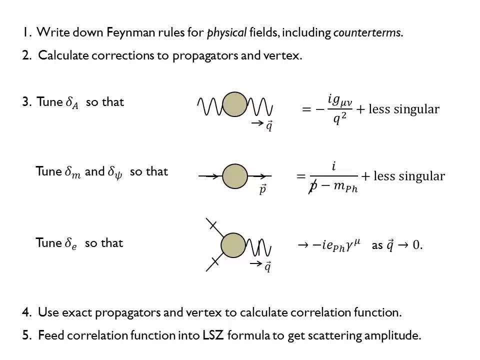 Finally, there is a requirement on the QED vertex, and that's quite subtle. The physical electron charge is a quantity that is essentially defined by a classical experiment, where you take a pair of charged boards, measure the force between them, and deduce the charge on each side. In this classical experiment, 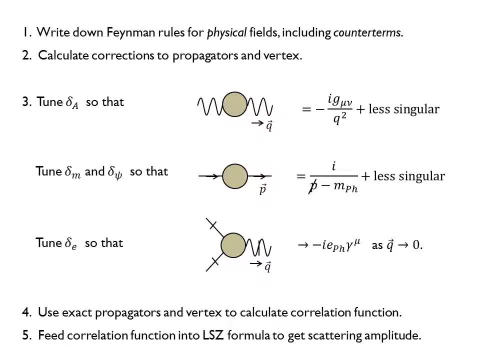 the momentum imparted from one board to the other is extremely small. 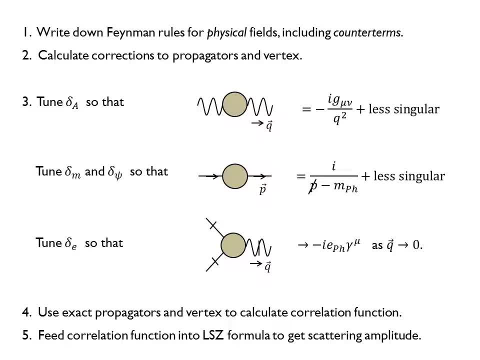 Now, our exact QED vertex, however complicated it may be, must reproduce the results of this classical experiment in the classical limit. 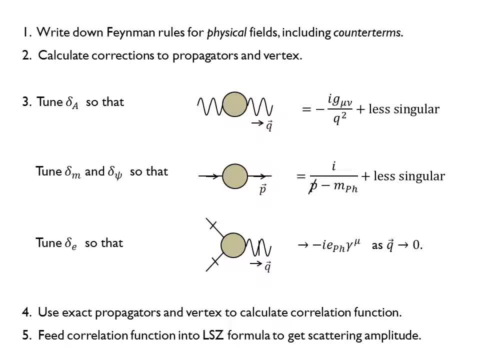 And you can show that this will be achieved if the vertex reduces to simply minus I times E physical times the gamma matrix 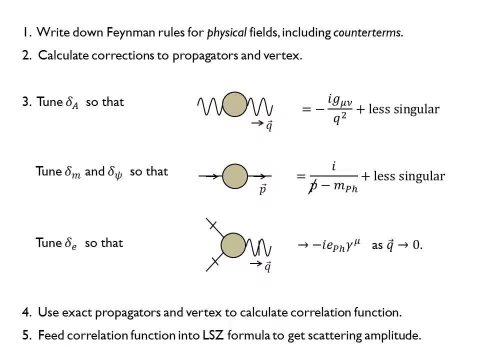 in the limit in which the momentum carries on. So you have to tune the counter term delta E to make this condition satisfied, 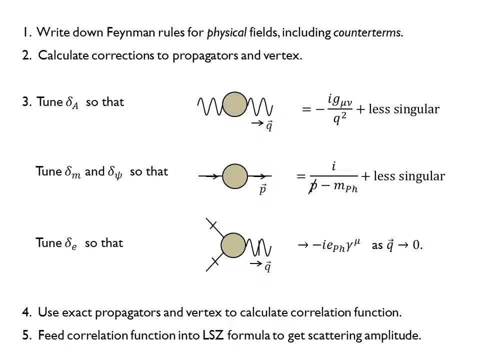 and that will ensure that the parameter E physical really is the physical charge on an electron. Once you have computed loop-order corrections to the propagators and the vertices, you can use them to work out scattering amplitudes. This procedure always gives finite answers in QED, 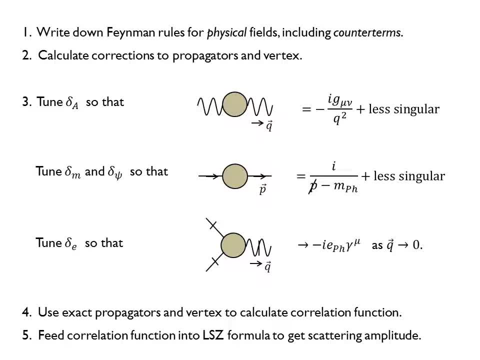 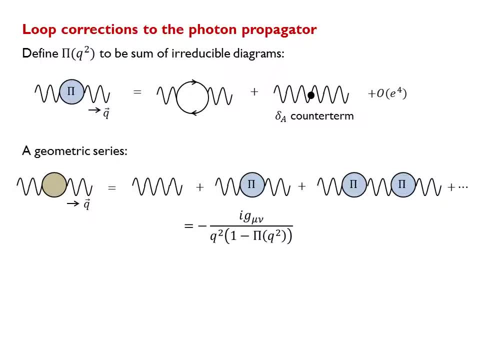 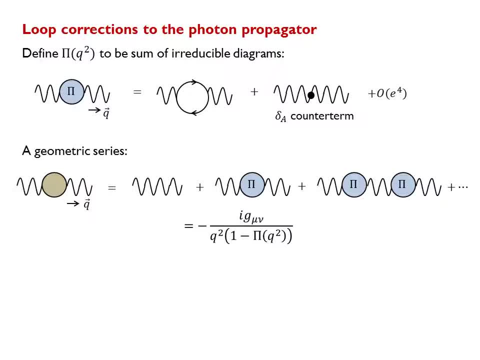 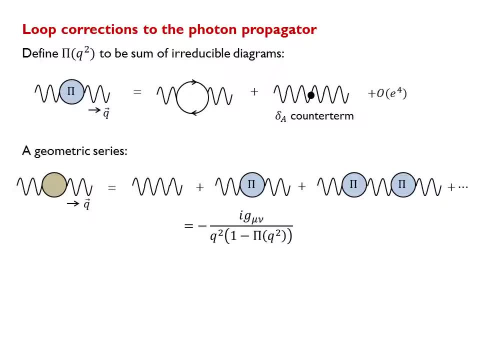 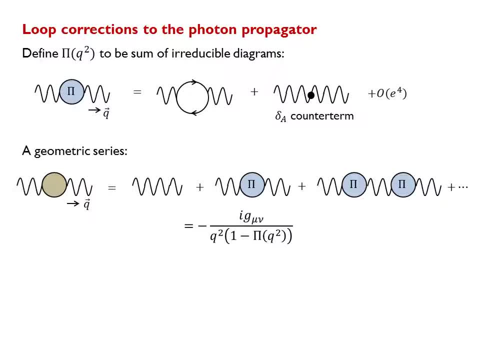 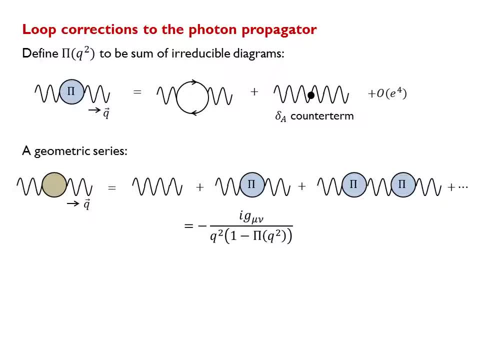 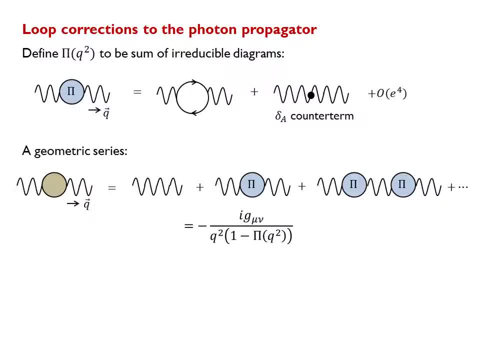 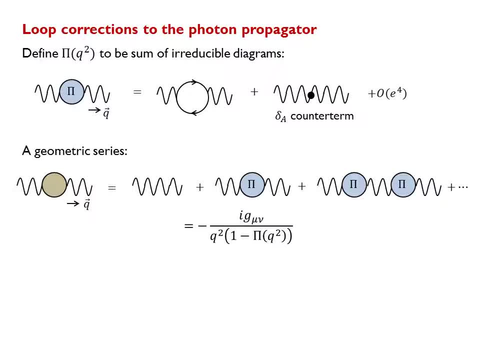 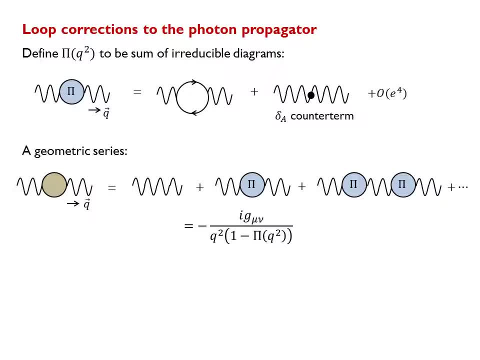 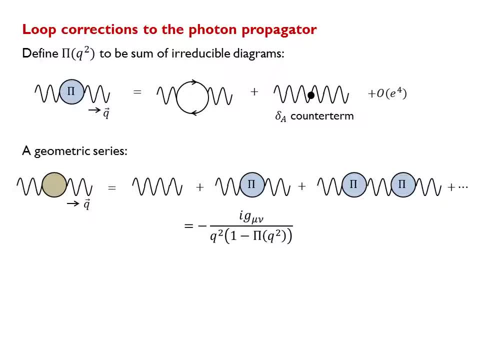 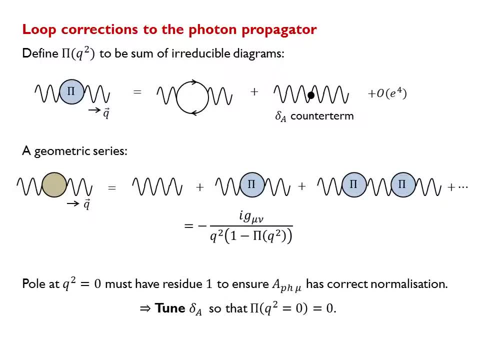 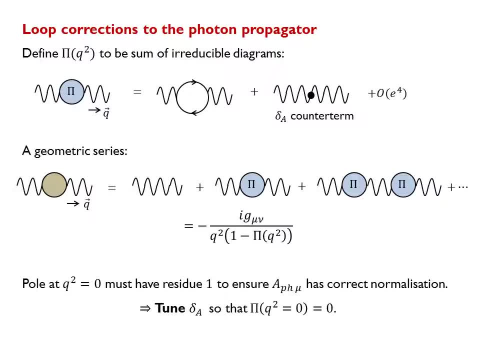 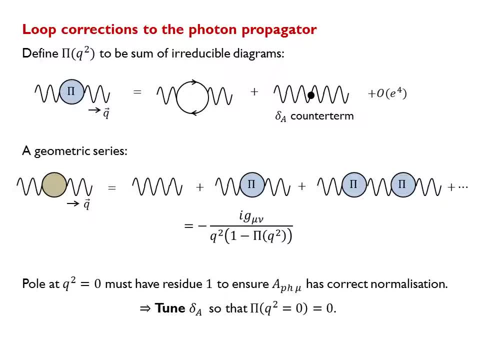 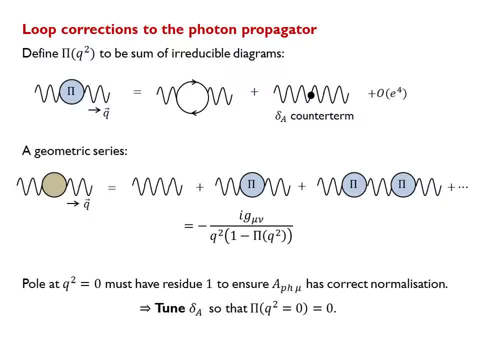 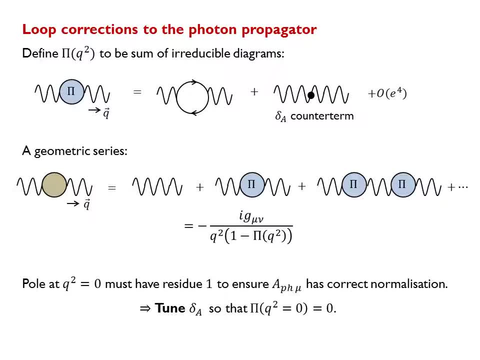 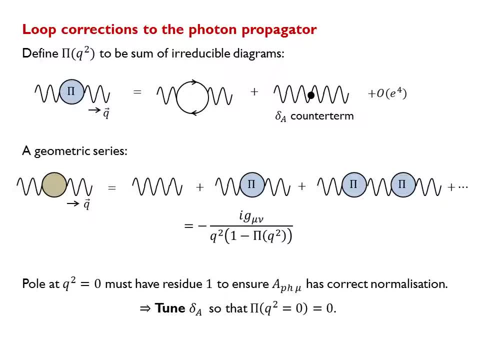 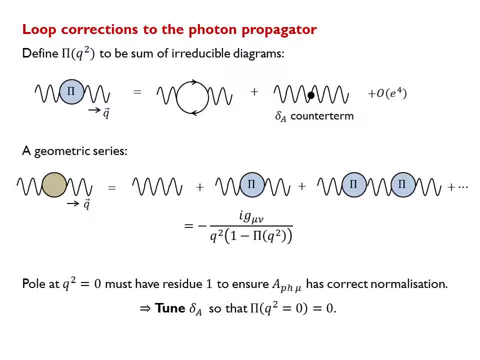 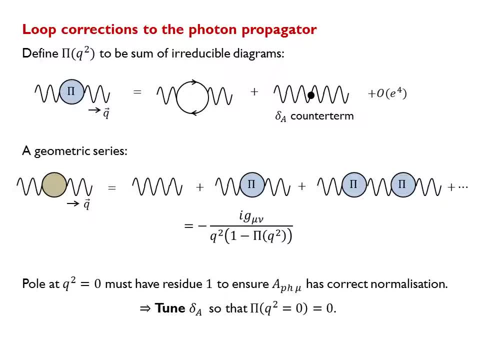 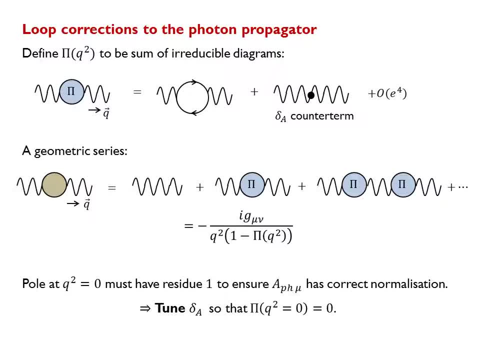 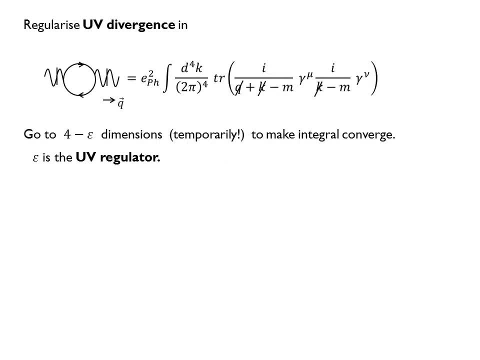 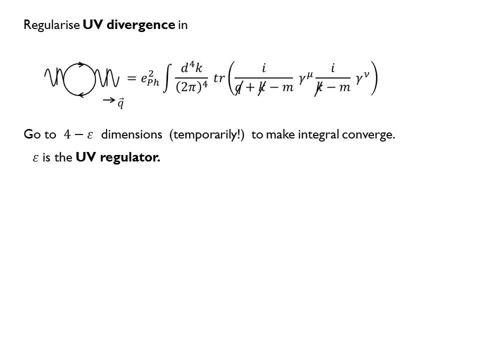 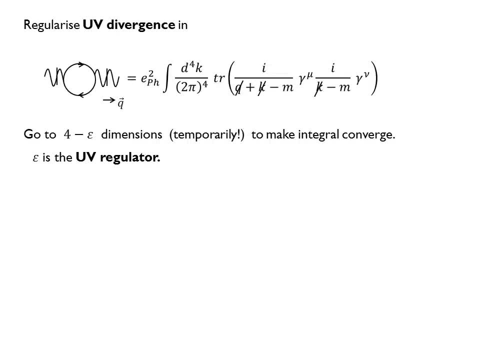 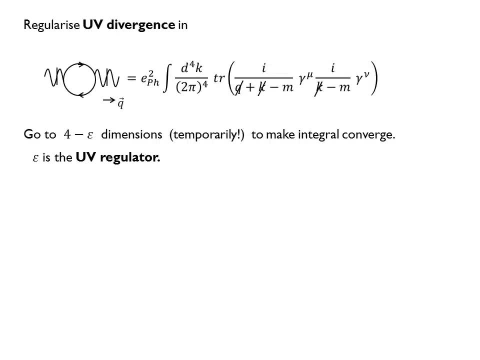 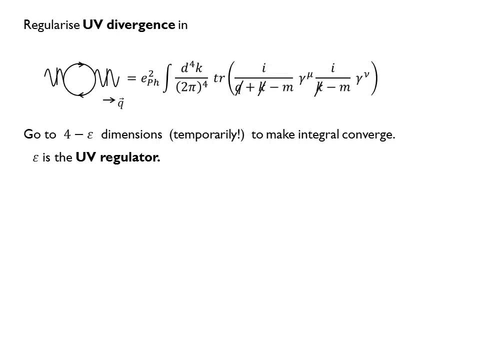 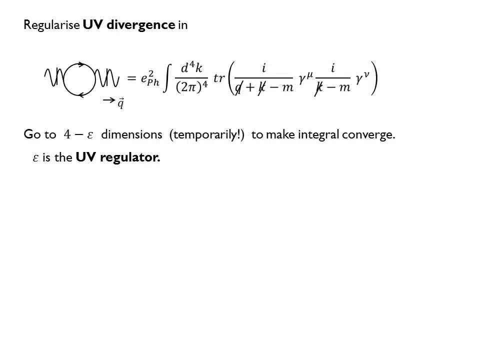 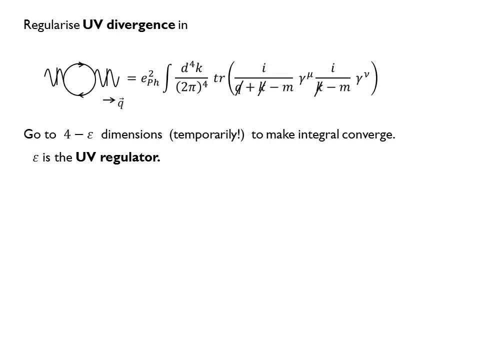 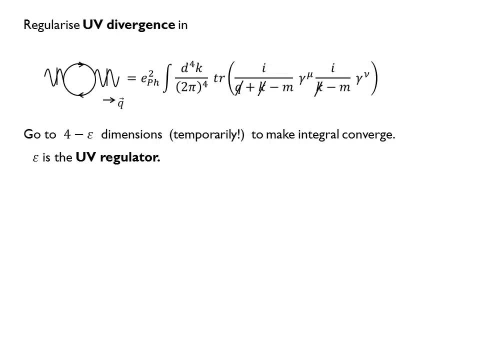 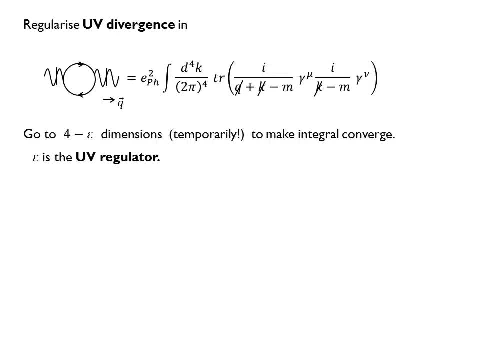 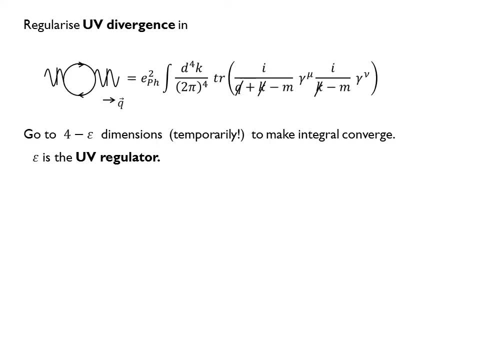 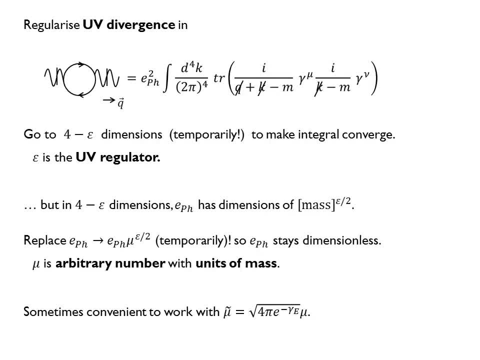 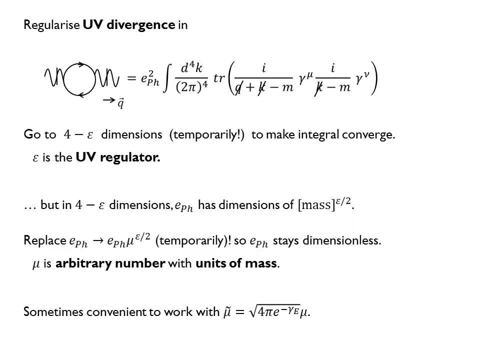 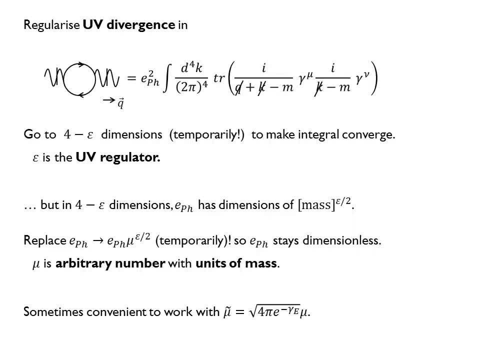 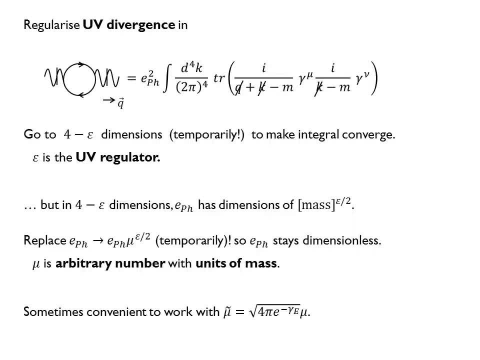 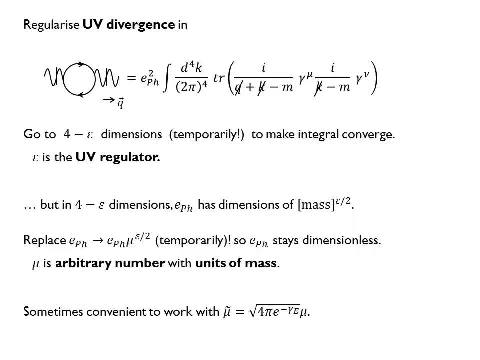 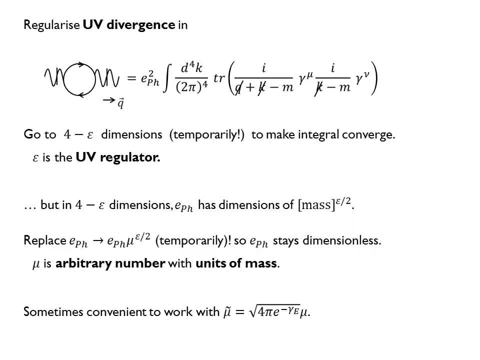 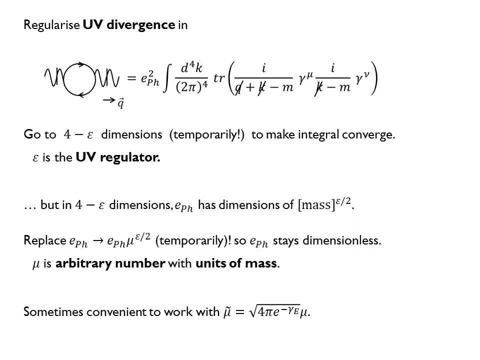 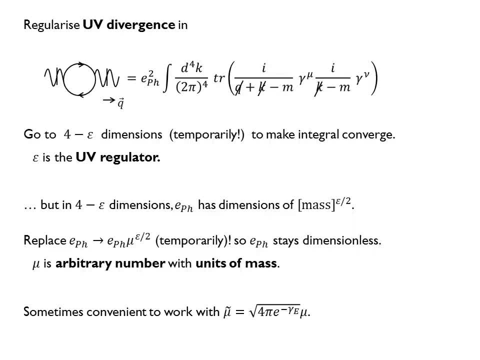 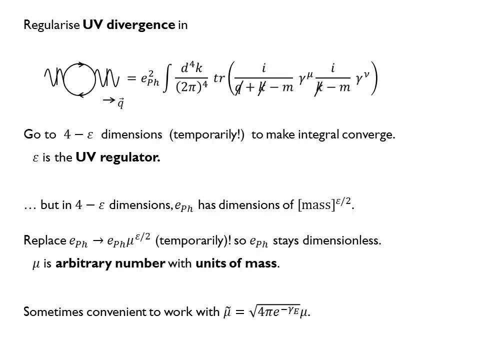 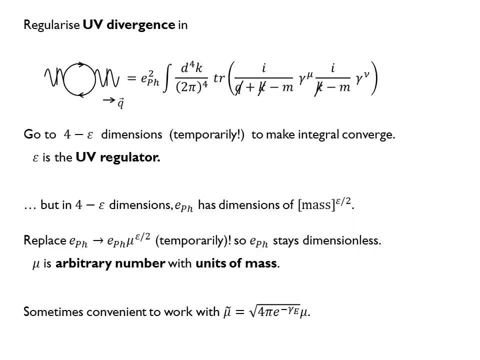 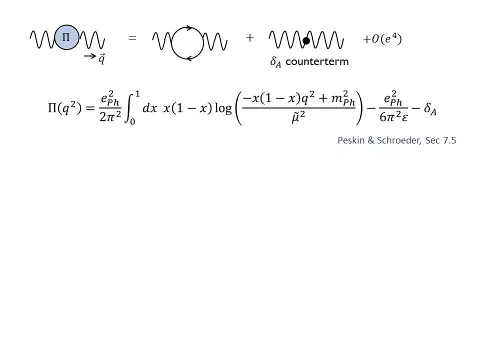 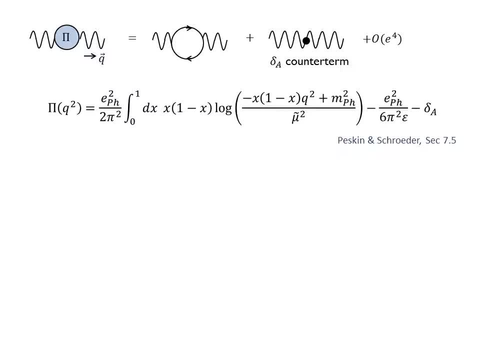 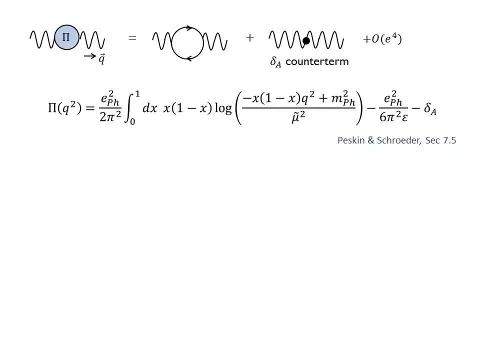 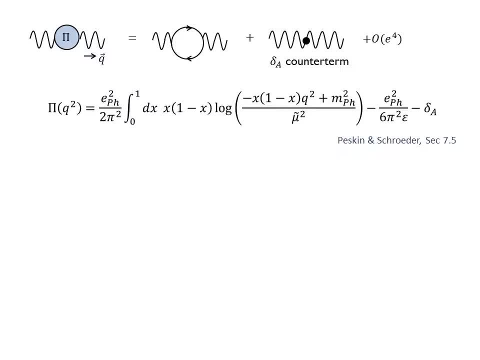 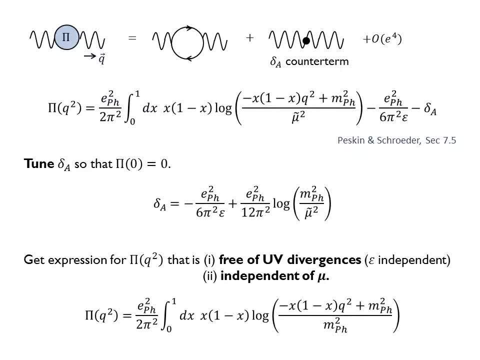 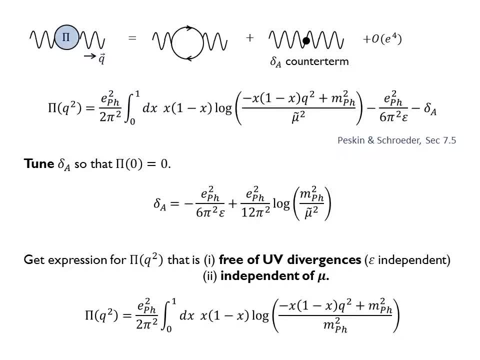 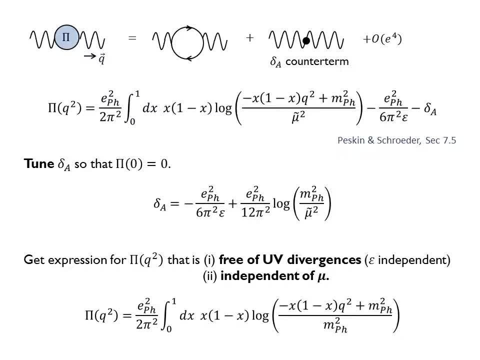 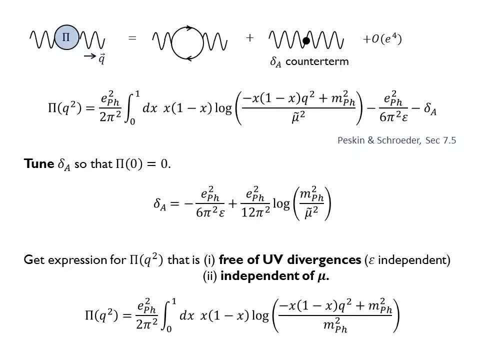 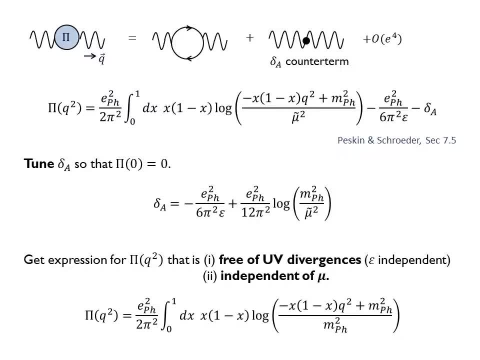 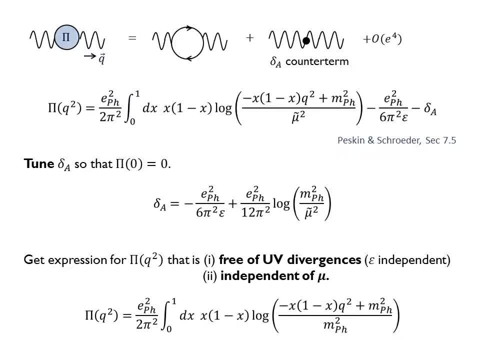 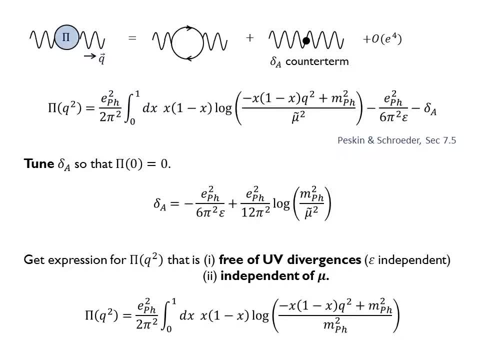 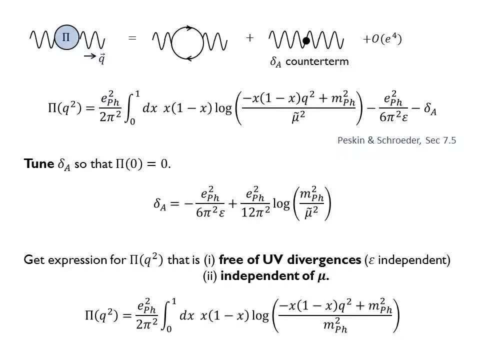 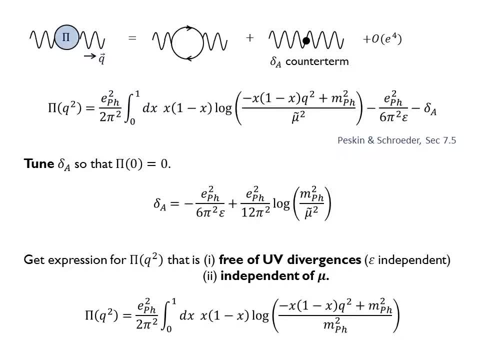 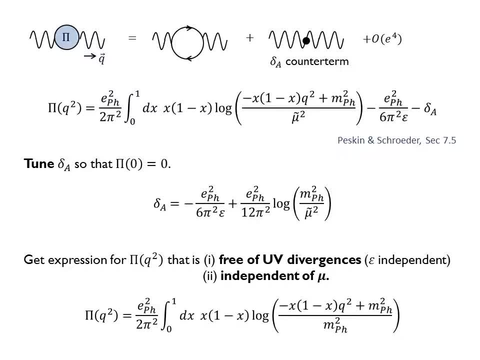 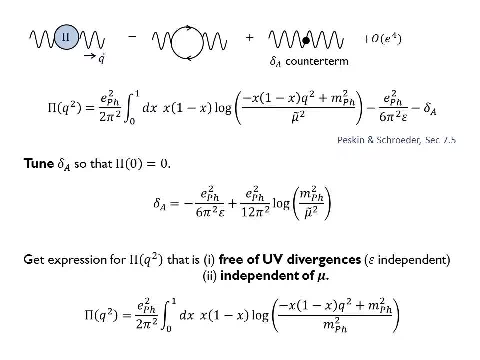 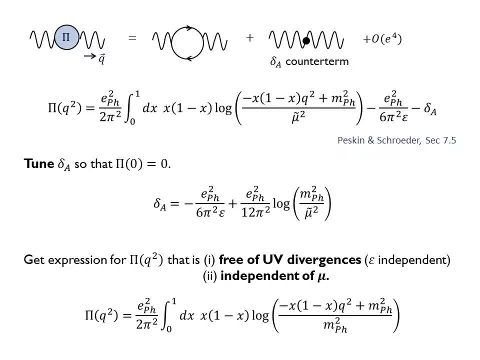 Yet this in itself was enough to resolve the problem about the UV divergence. 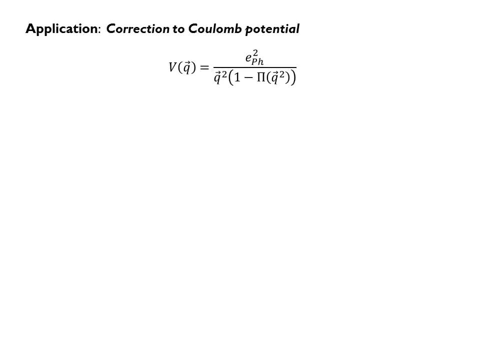 The photon propagator is an important quantity because it determines how the electromagnetic force propagates over different distances. In other words, it determines the Coulomb potential. And what we've just calculated is the QED correction to the Coulomb potential. 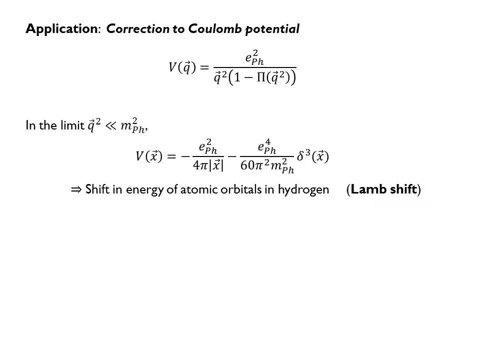 At small momentum, our calculation reproduces the classical Coulomb potential, but it adds a correction of order e to the 4 in the form of a delta function. This correction alters the energies of the electron orbitals in atoms. But only the s orbitals, which are the orbitals that penetrate to the nucleus and field this delta function. 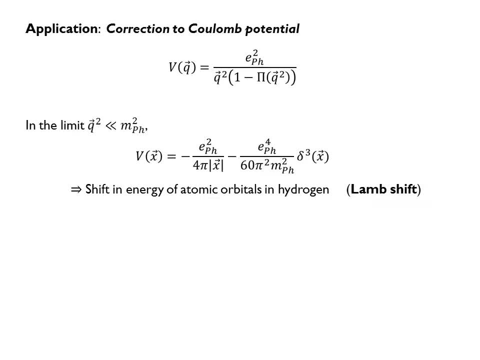 This effect has been measured and is considered to be one of the precision tests of QED. 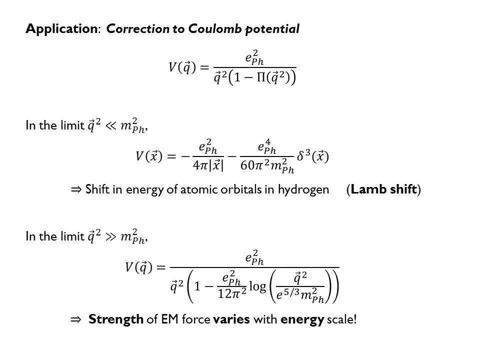 At large momentum, the Coulomb potential has a log dependence on Q. 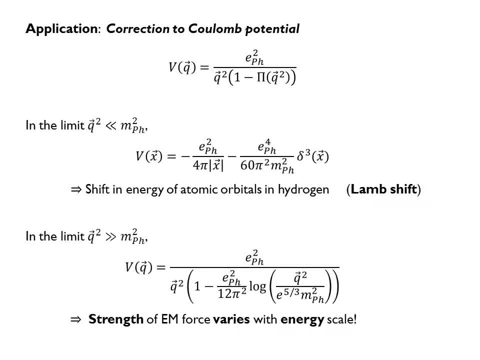 This is telling us that as momentum increases, the electromagnetic force becomes stronger. And this is a famous property of quantum electrodynamics. 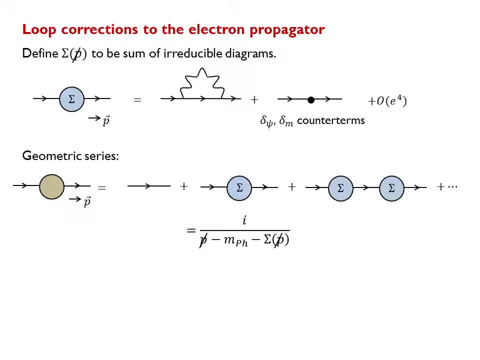 Loop corrections to the electron propagator can be worked out in pretty much the same way as for the photon propagator. There are two irreducible diagrams to consider. A photon loop diagram and a counter term diagram. As before, you can sum up all the loop corrections as a geometric series, and you end up with the expression i over p slash minus m physical minus the irreducible diagrams. We have to meet two conditions this time, namely that the pole of the propagator must be at p slash equals m physical, and the pole must have residue 1. 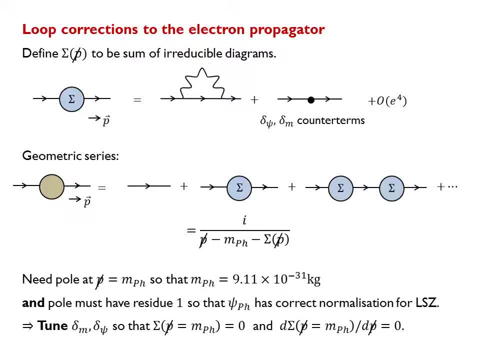 This is to ensure that m physical really is the physical mass of the electron, and to ensure that psi has the right normalization. 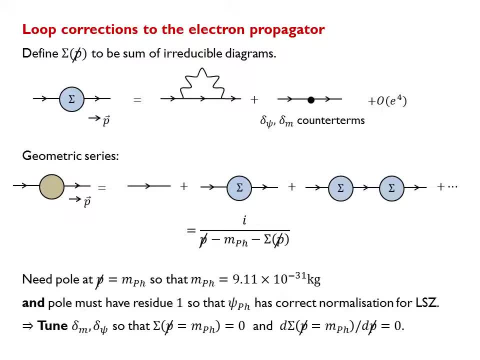 We have to tune both of these counter terms at the same time to meet both of these conditions. 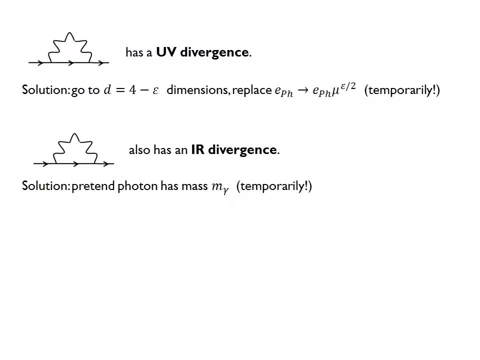 The diagram with a photon loop is particularly annoying because it has a UV divergence and an IR divergence. We can regularize the UV divergence as we did before, by reducing the number of dimensions in the theory to make the integral converge, and then introducing an arbitrary mass scale to keep the coupling constant dimensionless while we do this. So where does the IR divergence converge? It comes from the fact that the photon is massless, and the integral of a massless propagator over momentum space is infinity. 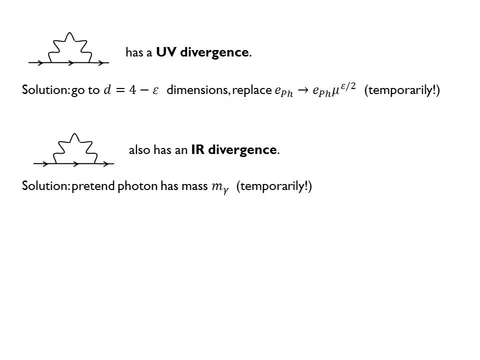 So to get around this obstacle, we're going to give the photon a fake mass, m gamma. 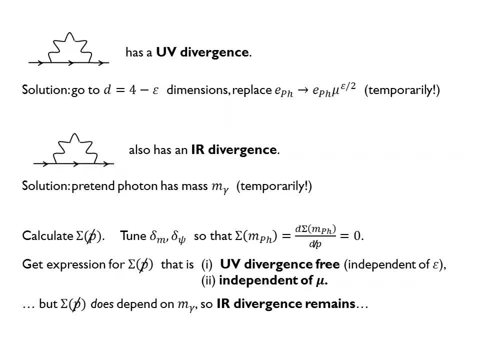 As before, we can go ahead and compute the loop corrections using the Feynman rules, tuning the counter terms to meet the normalization conditions. I decided not to put up the final formula, not to put up the final expression for the propagator on the slide, but suffice it to say that the one-loop electron propagator is free of UV divergences, and is independent of the arbitrary mass scale, mu. 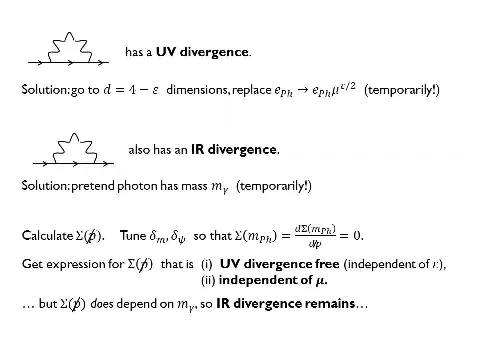 Just like the photon propagator, all of the epsilon and mu dependents have been absorbed into the counter terms. However, the electron propagator does explicitly depend on a fake photon mass, so the IR divergence remains, and this is something we'll have to confront later. 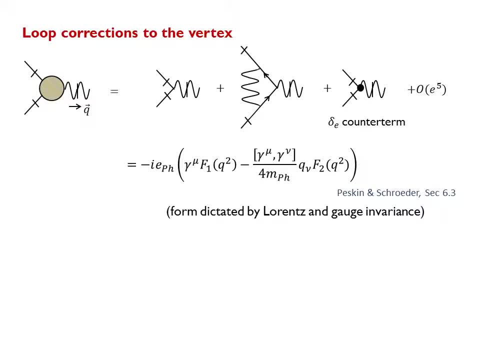 The vertex correction is very similar. There's a loop diagram to consider, and there's a counter term diagram. It turns out that Lorentz and gauge symmetries fix the overall structure of the QED vertex, and all the non-trivial information is contained inside two functions, f1 and f2, which we have to compute using Feynman rules from those diagrams. 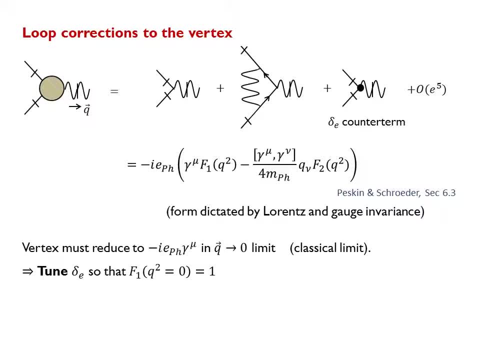 The condition that we want to impose on the vertex is to ensure that E physical really is the same thing as the electric charge measured in the classical Coulomb law experiment. And the condition is that the vertex reduces to minus I times E physical times the gamma matrix in the limits as the photon momentum goes to zero. 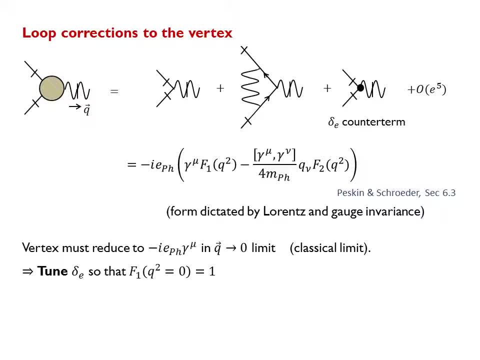 And we do that by tuning delta E so that f1 equals 1 when Q squared equals zero. 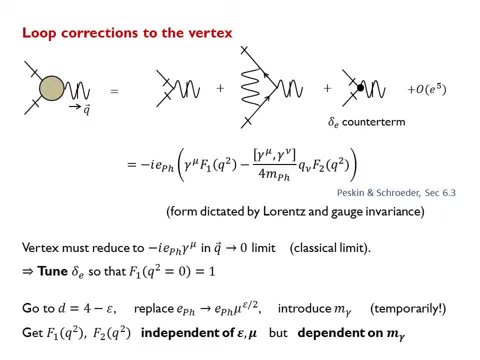 Like for the electron propagator, there are UV divergences and there are IR divergences, and we're going to deal with them in a usual way. 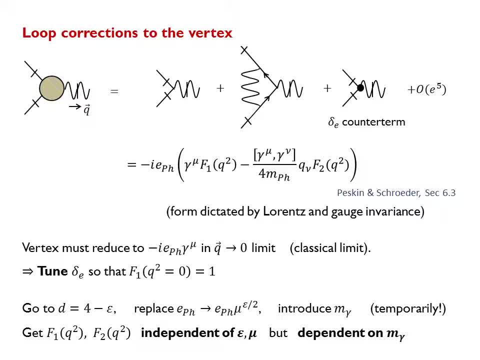 If we follow the procedure again, we're going to get functions f1 and f2 which are independent of epsilon and mu, but are dependent on a fake photon mass. 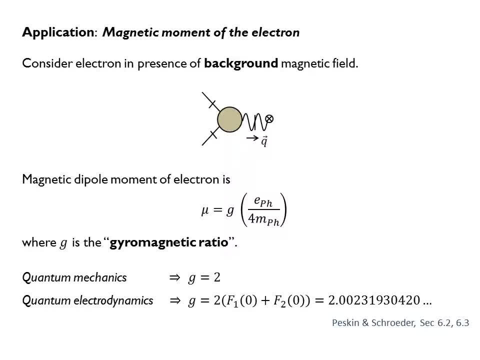 The QED vertex tells us about how electrons interact with gauge fields, and it has an incredibly famous application, which is that it predicts the magnetic dipole moment of the electron. 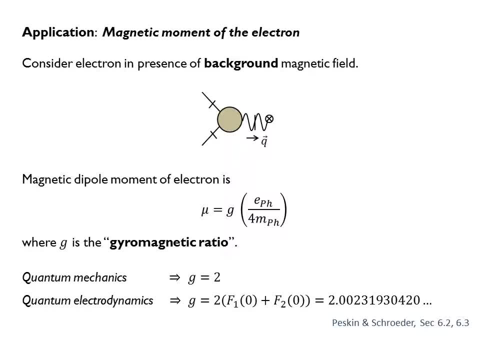 This calculation all boils down to evaluating a dimensionless number called the gyromagnetic ratio, G. 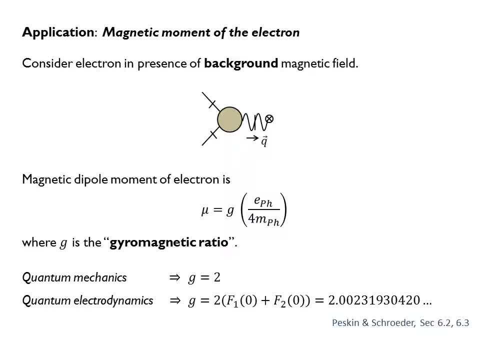 Now quantum mechanics says that G is exactly 2, and you probably did that in your undergraduate studies. 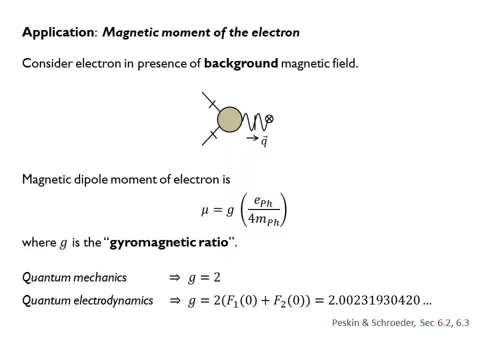 But quantum electrodynamics says that G is determined by those two functions, f1 and f2, in the exact vertex. 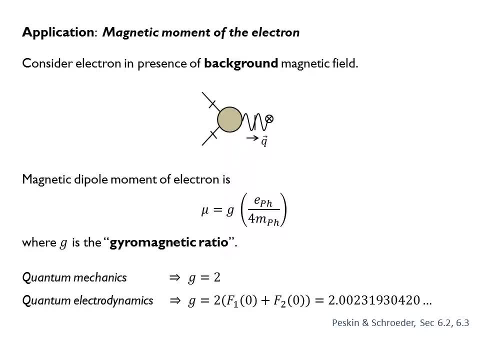 This has been worked out to several orders in perturbation theory, and the answer that you get from quantum electrodynamics agrees with experiments to 11 significant figures, which makes it the most accurate prediction that's ever been made. 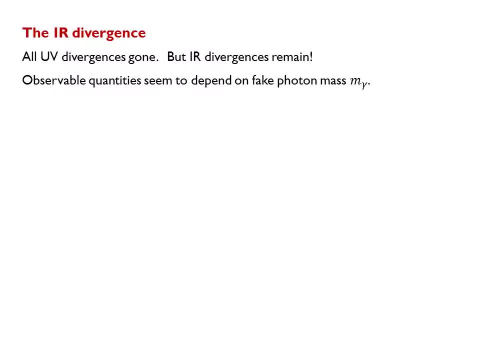 So as far as the UV divergences are concerned, we're done. Now let's deal with the IR divergences in the same way, not by inventing an artificial means of removing them, but by carefully questioning our physical analysis. And the way to do this is incredibly neat. 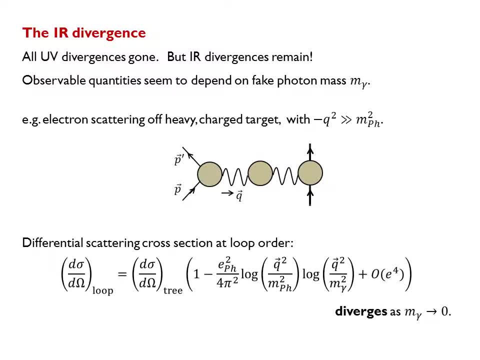 Let's use this as our example, an electron scattering off a heavy target. The observable quantity that you would measure in this experiment is called the differential scattering cross-section, and this is the probability of the electron being scattered at a particular angle when it hits the target. 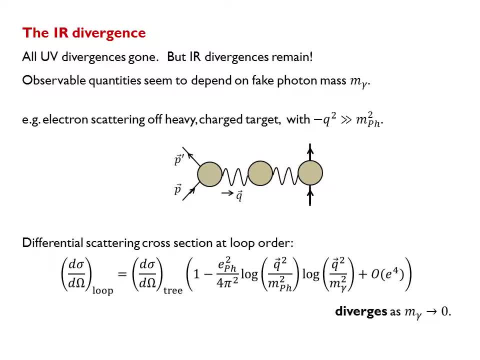 You can calculate this quantity to loop order using the corrections to the vertex and the propagators that we derived on the earlier slides. 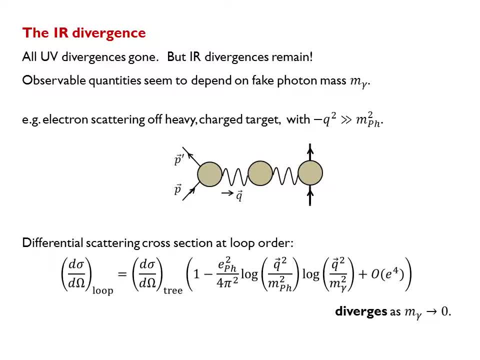 And if you do this, it reduces to the simple expression that I've written here. The trouble with this expression is that it depends explicitly on a fake mass that we gave to the photon to regulate the IR divergences, and this cross-section blows up if you try to take the cut-off away. 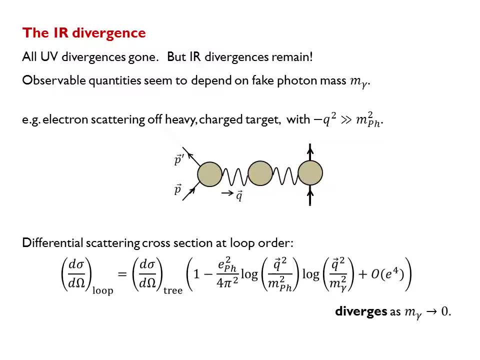 This is telling us that there's a mistake somewhere in our analysis. The subtlety that we've missed is that this scattering process doesn't just happen on its own. 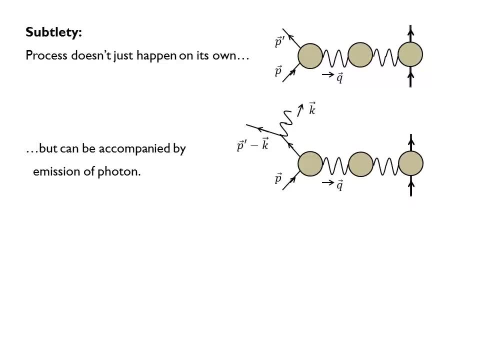 In addition to the scattering process itself, it's possible for the outgoing electron to radiate a photon. Although you might consider the photon radiation to be a different process, you have to ask yourself whether the detector in this experiment can actually tell the difference between the two processes. Because if the extra photon has very low momentum, then the electron will radiate at a different rate and if the extra photon has very low momentum, then the photon won't be recorded by the detector and the emission of the photon won't cause any noticeable deviation in the trajectory of the electron. 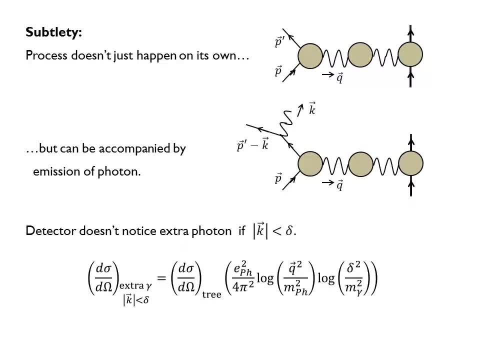 So as long as the extra photon has momentum less than delta, say, where delta is a property of the detector, the detector can't tell the difference between the two processes, and we should include the scattering cross-section for the process with the photon emitted as our answer. 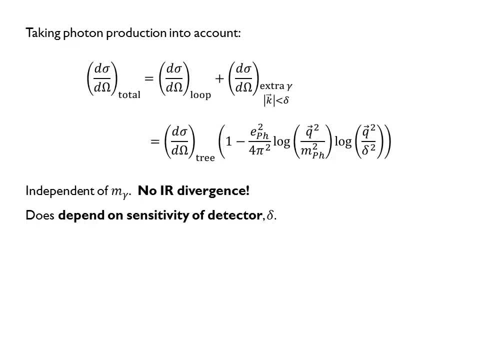 The scattering cross-section of the original process depends on the fake photon mass. The scattering cross-section of the process with an extra photon produced also depends on the fake photon mass. 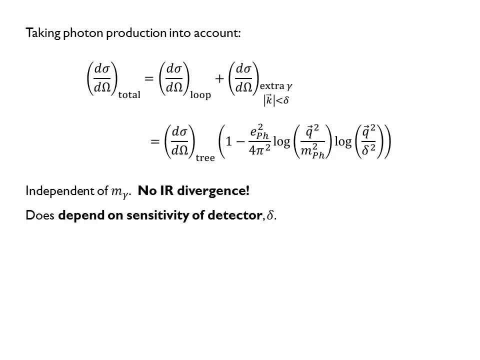 But when you add the two processes together, the dependence on the photon mass cancels out. So the sum of the two contributions has no IR divergence. 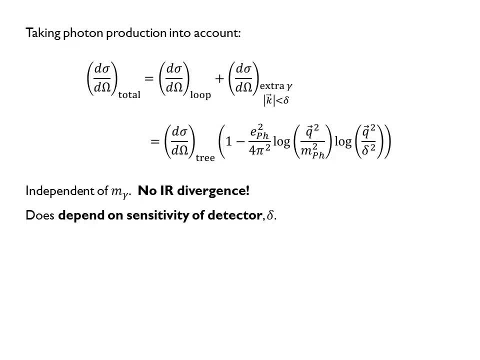 The answer depends only on the physical charge, the physical mass of the electron, and the sensitivity of the detector. 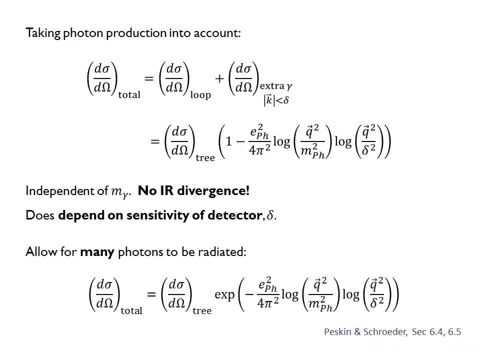 When you allow for the emission of more than one photon, this correction factor that multiplies the tree-level result turns into an exponential. 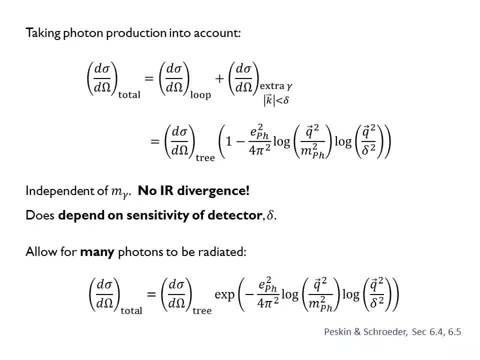 Notice that in the limit as delta tends to zero, which is when you have a perfectly sensitive detector, this cross-section tends to zero. This is telling you that the scattering process never happens by itself. It is always accompanied by the emission of photons. And that is the physical insight required to handle this IR divergence. 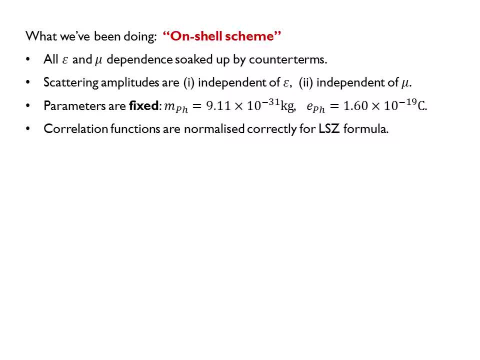 Up until now, we've been following a procedure called the on-shell renormalization scheme. 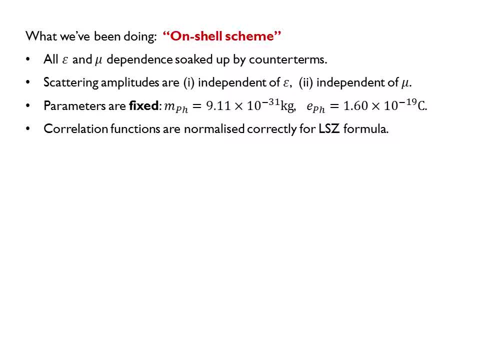 This is a scheme where physical predictions are expressed in terms of fixed physical parameters. The UV regulator epsilon and the arbitrary mass scale mu get absorbed by the counter terms, leaving no arbitrary parameters in the final answers. 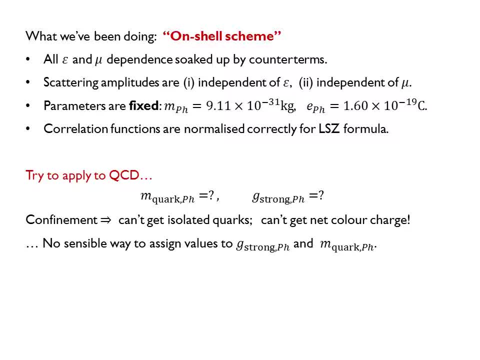 So what happens if we try to apply this procedure to quantum chromodynamics? Immediately, you hit a conceptual problem. What value are you going to assign for the mass of a quark? Well, you can't assign one because you can't measure a quark on its own. Quarks are always bound inside baryons and mesons. And what value are you going to assign to the QCD coupling? You don't know because you can't do the analogue of the classical Coulomb law experiment with a strong force. 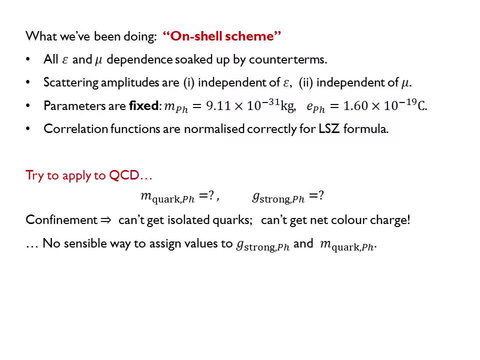 And with no asymptotic particles, the LSZ normalization condition doesn't make any sense either. 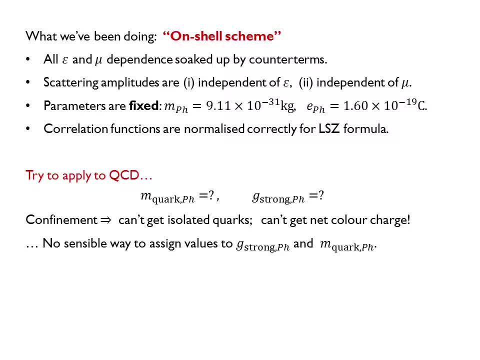 So when it comes to QCD, we're forced to abandon the on-shell scheme and try something else. 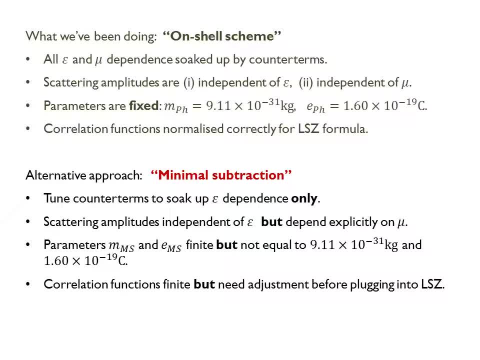 One of the popular alternatives is called minimal subtraction. Like the name suggests, this is a scheme where the counter terms are tuned to soak up just the divergences and leave behind everything else. 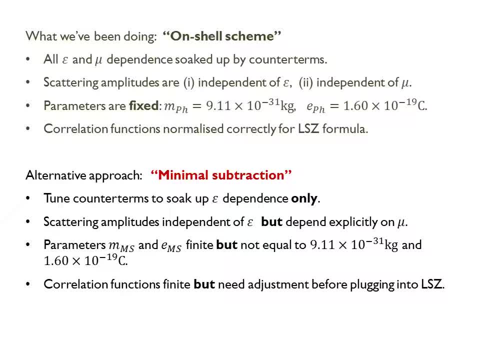 What is left behind is a scattering amplitude that is finite but depends on the arbitrary mass scale mu. And it'll be expressed in terms of parameters that are finite but not equal to any particular privilege values. 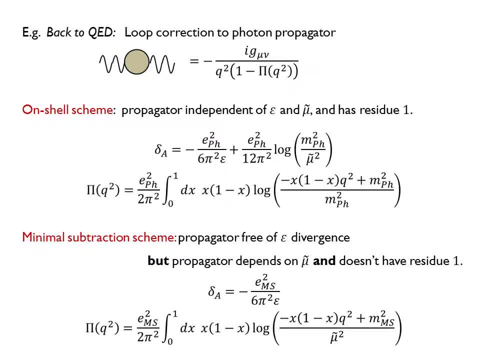 It's best to explain this using an example, so let's go back to QED and compare the two schemes in the case of the photon propagator. 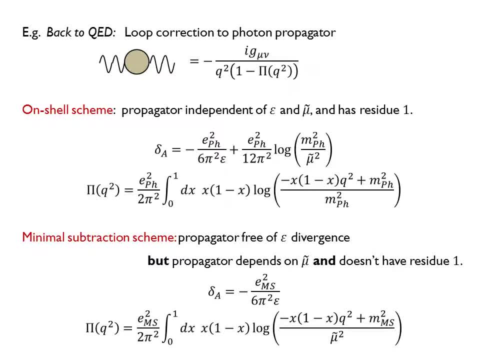 In the on-shell scheme, the counter term automatically soaks up the epsilon and mu dependence, and you're left with a propagator that depends just on the physical electron mass and the physical unit of electric charge. Also, the propagator has residue 1, which is good. 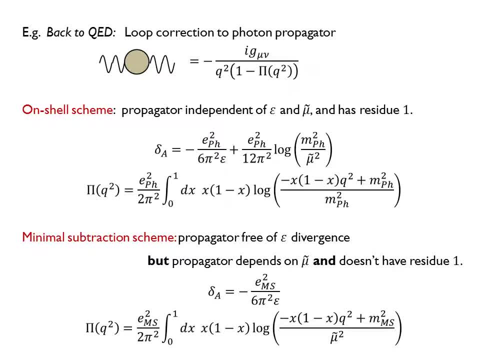 In the minimal subtraction scheme, the counter term is chosen to be the minimum subtraction. 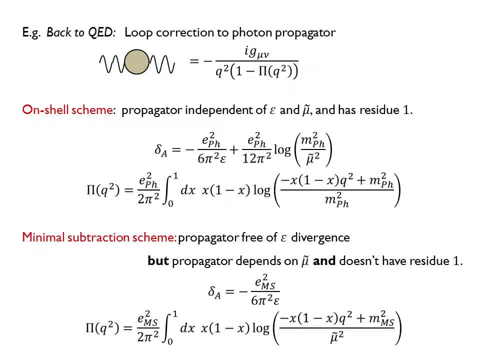 Just to strip off the UV divergent term, which is the term containing 1 over epsilon. 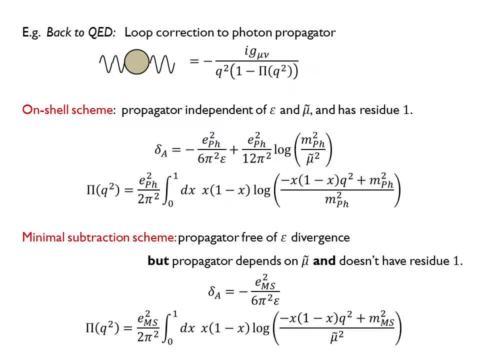 That leaves behind a propagator that depends explicitly on the arbitrary energy scale mu. And this propagator is expressed in terms of charge and mass parameters that are finite but are not the privileged ones 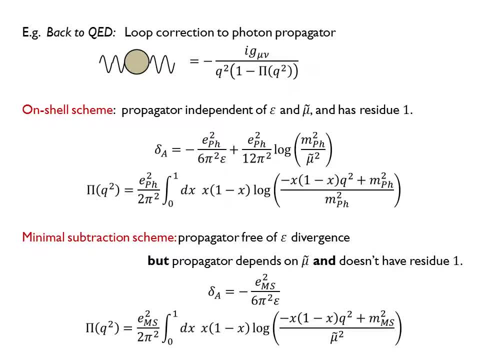 1.6 times 10 to the minus 19 coulombs and 9.1 times 10 to the minus 31 kilograms. 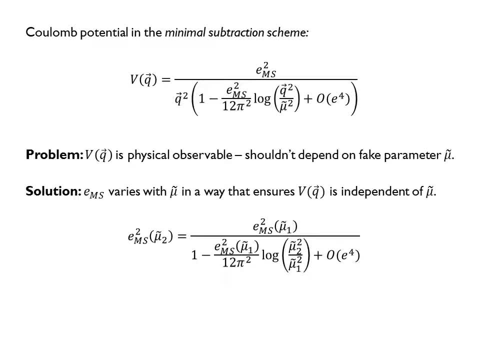 Let's also look at what the minimal subtraction scheme gives us for the coulomb potential. The coulomb potential is a physically observable quantity, and it looks like it depends on the number mu. 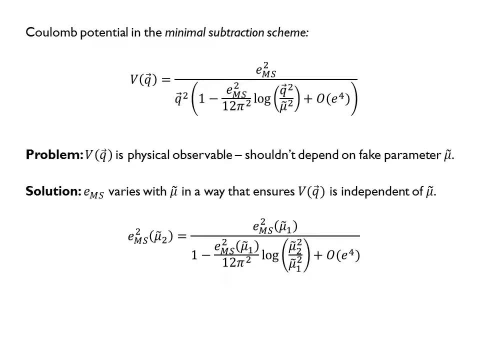 But mu is not a genuine parameter, it's just a made-up number that we introduce in the middle-of-hour calculation. So the coulomb potential shouldn't depend on mu. 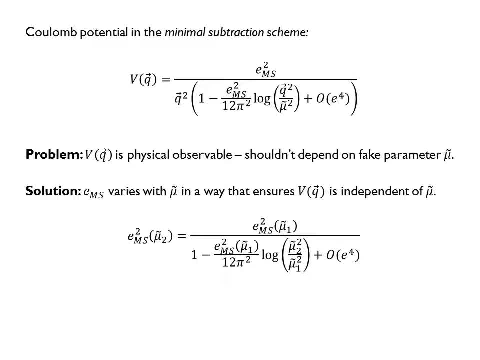 The solution to this conundrum is that for every value of mu, the coupling constant itself makes a different value. 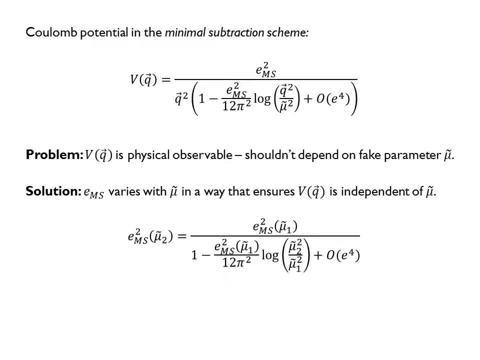 And the way in which the coupling constant varies with mu should cancel out the explicit mu dependence in V. 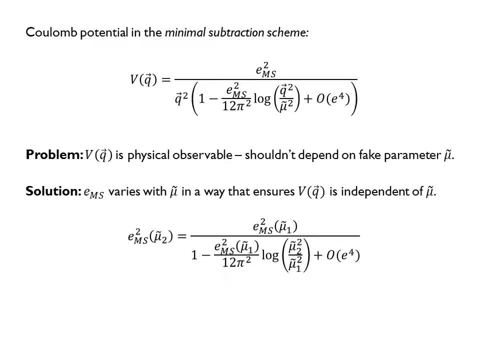 And if we work out how the coupling constant varies with mu, this is the expression that you get. 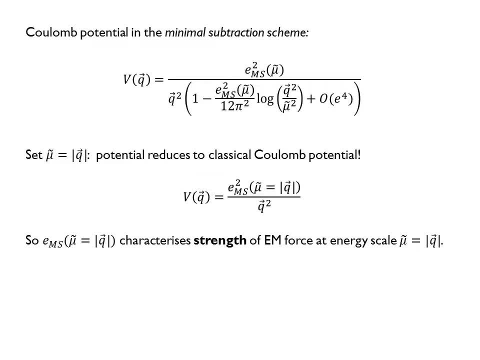 Look what happens if we set mu equal to the momentum q at which the coulomb potential is evaluated. 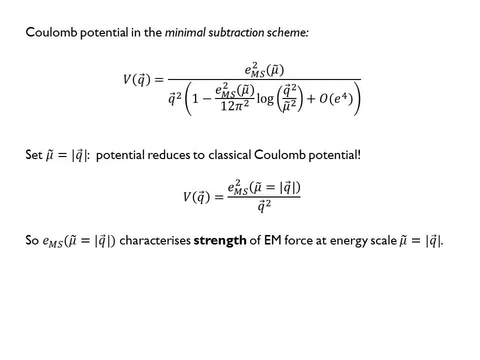 The log disappears, and all you're left with is something that looks like the classical coulomb potential, except... 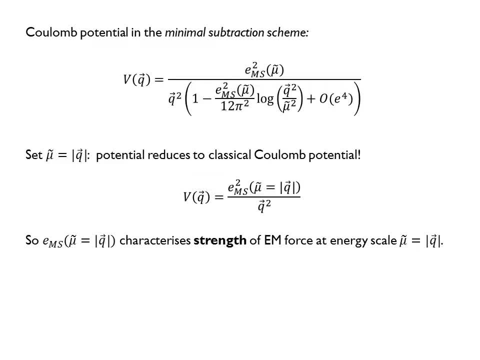 that the coupling constant in the numerator isn't the classical charge 1.6 times 10 to the minus 19, but it's the minimum subtraction charge parameter at scale mu equals q. 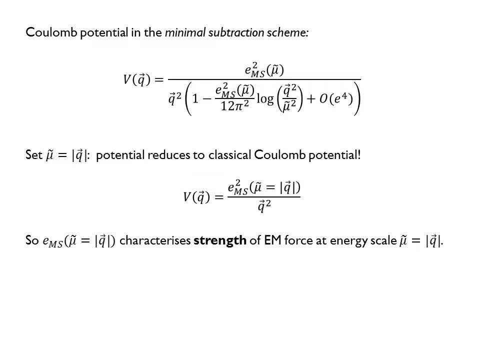 And that's why people say that the value of the coupling constant at scale q determines the strength of the interaction at energy q. 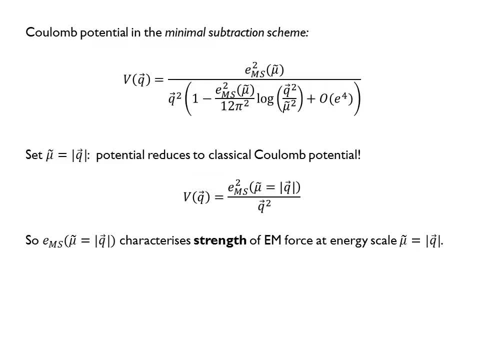 Because of this observation, you shouldn't think of the mu dependence of the coupling as a nuisance. 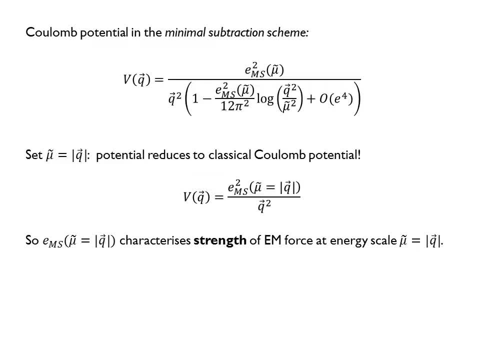 It's actually telling you something useful about how the interaction gets stronger or weaker at different energies. 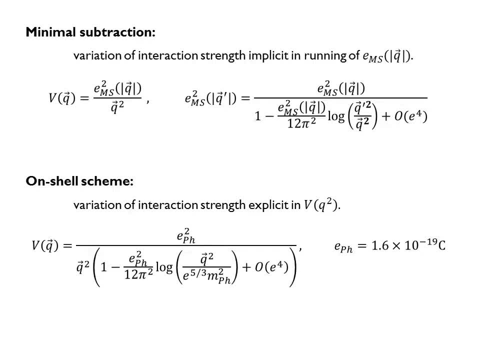 That is not to say that the energy dependence of the interaction only shows up in the minimal subtraction scheme. It also shows up in the on-shell scheme, where the coupling constant is fixed, but the energy dependence is made explicit in the expression for V. 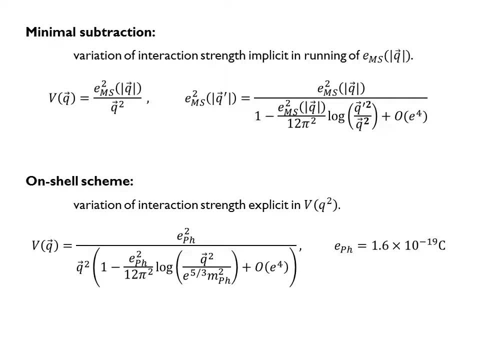 So you can think of the two schemes as different accounting procedures that give you the same answers in the end.